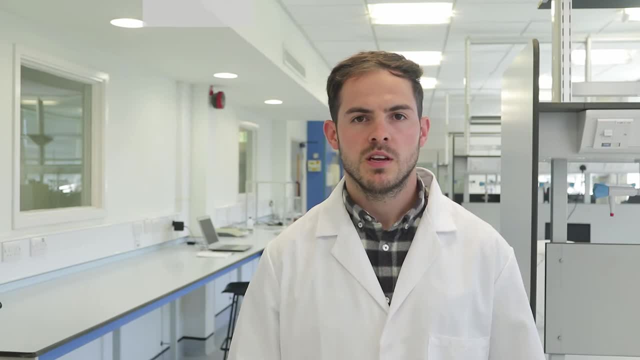 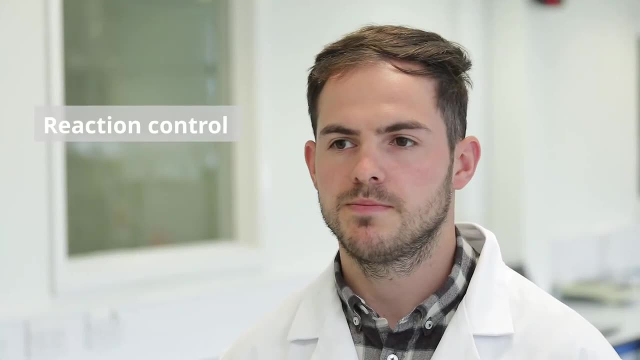 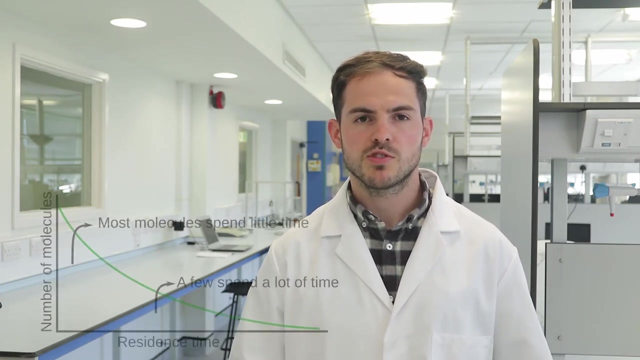 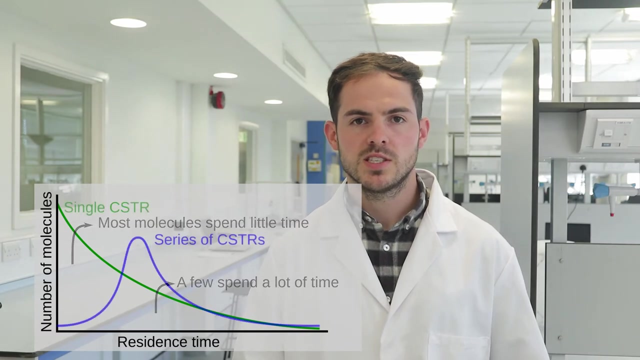 are common and are comparatively cheap to construct. However, scaling up requires some investment in research and piloting. How well can you control the reaction? A single CSTR suffers from relatively slow heat and mass transfer. Also, residence time control is poor. does not necessarily flow through the reactor at the same rate, but a series of CSTRs can. 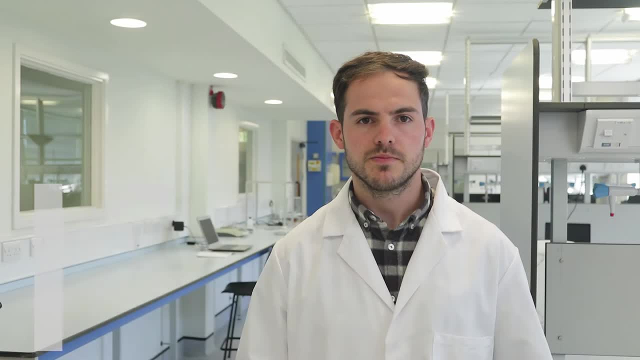 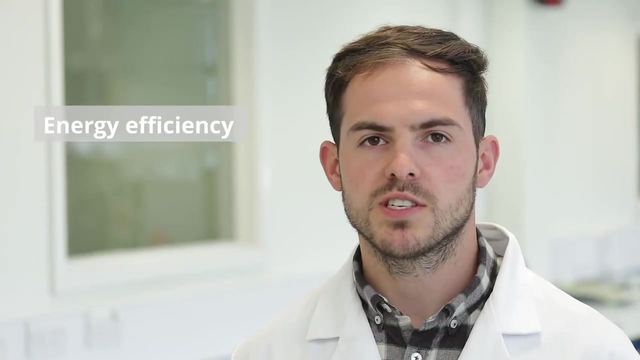 be connected for better control over residence time. Agitation is a really important part of the CSTR. A variety of stirring impellers are available. However, even with the best impellers, dead zones where no mixing occur will still exist. What about energy efficiency? CSTRs are more energy efficient than batch reactors. This 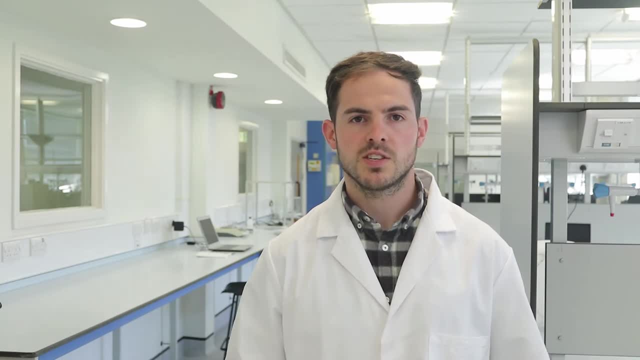 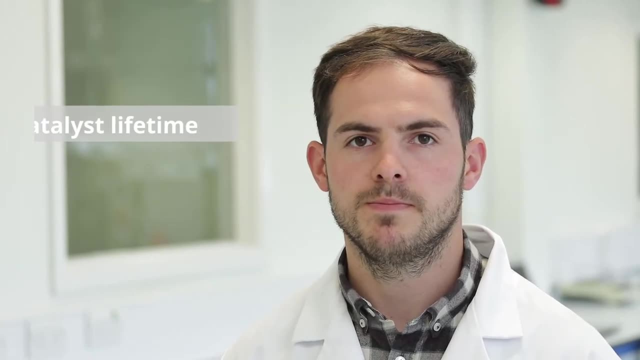 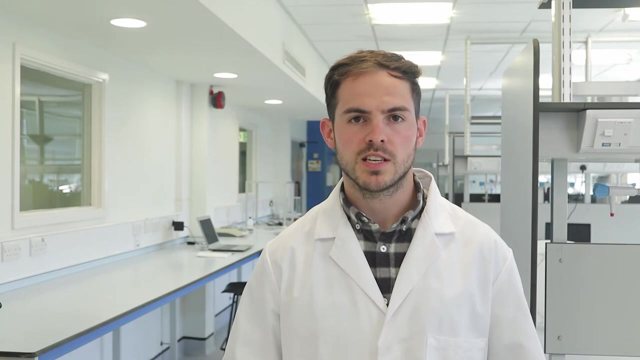 is because the reaction is continuous and there isn't the need to go through empty fill and heat up cycles. And lastly, for catalytic reactions, what is the catalyst lifetime? A wide range of catalysts can be used in CSTRs, such as heterogeneous catalysts which are solid catalysts in a 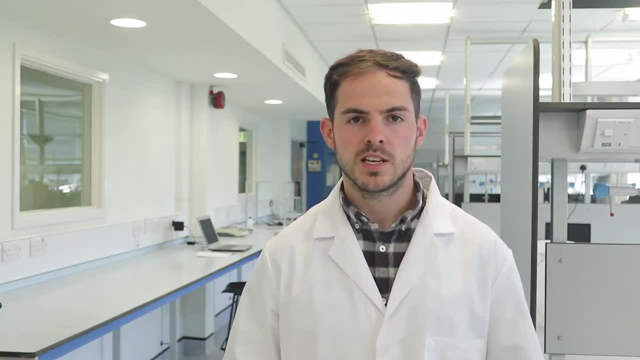 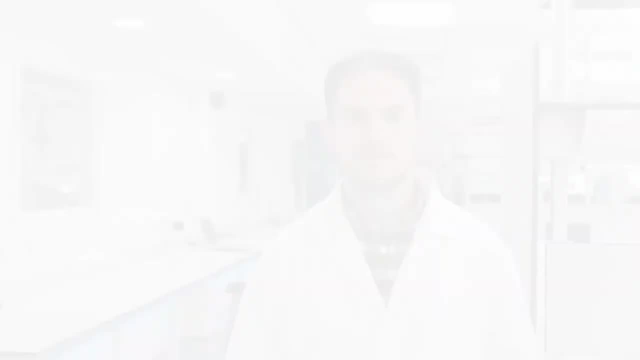 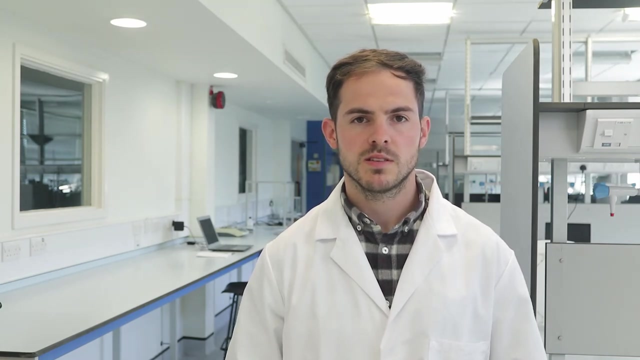 liquid reaction medium, homogeneous catalysts, where both catalyst and reaction medium are in the liquid phase, or even biological catalysts such as enzymes. Because of the continuous operation, the lifetime of the catalyst is not so limited by the reactor. compared to batch processes, However, because the catalysts are often small particles or even liquids. 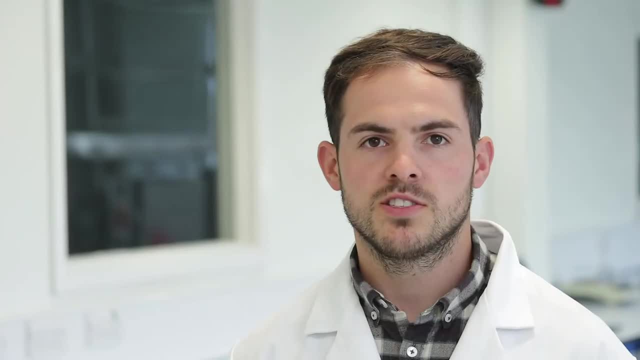 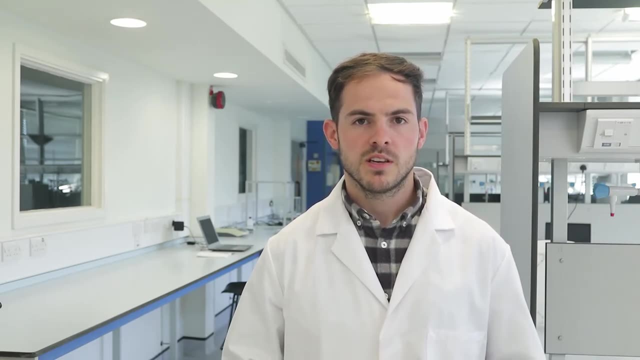 separation of the catalysts is still an issue. To summarise CSTRs: hopefully you have a better understanding of continuous stirred reactors now. We have given the reactor a subjective score based on our experience. Scope: The CSTR is excellent as a wide range of reactions can be carried out in them. 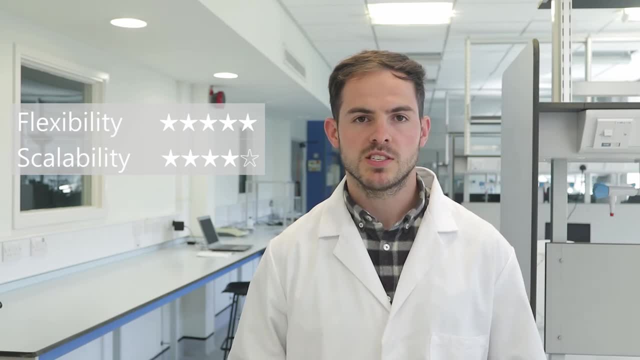 Scalability: Scalability is good. Again, this is similar to batch. There can be challenges, but these can be easily addressed. Reaction control: Reaction control is average. CSTRs do suffer from mass transfer limitations due to their geometry. In addition, residence times often have broad distributions because all molecules